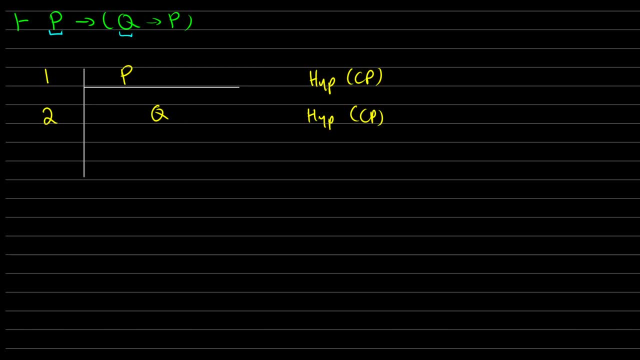 but then we have to assume q to do q arrow p. Okay, so in line three, let me set up this thing here. So we're going to need probably two lines there, which means I'll have to extend this out by one. Okay, in three I'm going to reiterate p from line one, So one. there's reiteration. 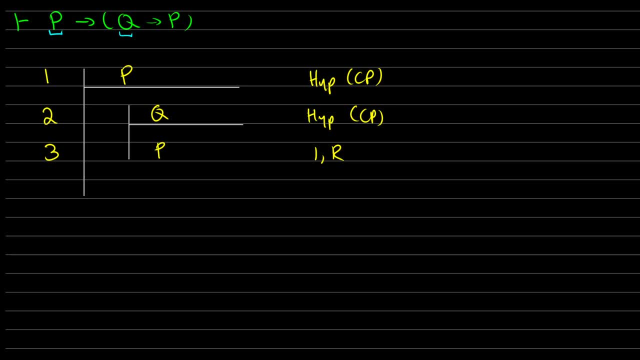 Okay, well, now we have a proof of q, or proof from q to p, line two to three, So we can pull q arrow p out in line four. so this is from two to three, a conditional proof. and now in line five, Well, we assumed- let me just make this a little bit nicer- we assumed: 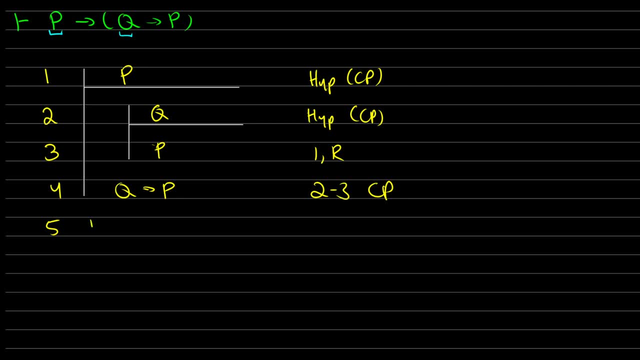 that we had p and we got q arrow p from it. so, using a conditional proof we now have: if p, then q arrow p. so that's from one to four and that's a conditional proof. Okay, that one, not too much trouble. That's pretty much it. so see you next time on Qarrow P, Qwp. Bye, bye. next time on Qarrow P, Qwp, Qwp, Qwp. next time on Qarrow P, Qwp, Qwp. next time on Qarrow P, Qwp, Qwp. next time on Qarrow P, Qwp, Qwp. 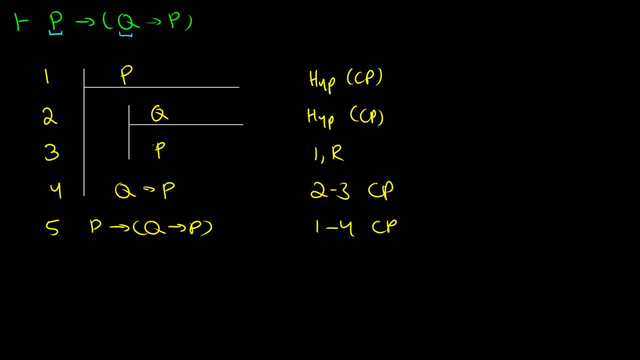 Not too bad. In fact, I think we've seen things very similar to this, but this is how we do p-arrow, q-arrow p, so we can use this any time that we want. Okay, this one. If we have p, then q, then r. then we have the fact that if p q, then p r. 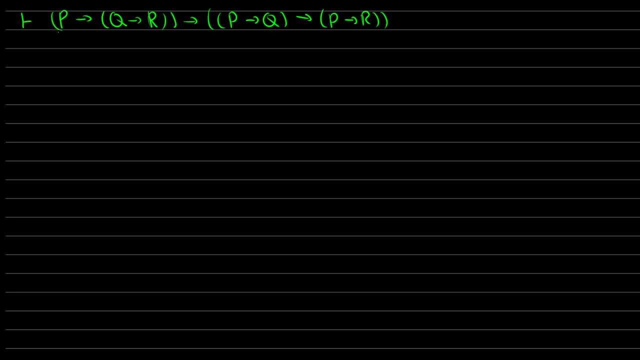 Okay. so this one a little bit longer, but the same idea. Okay, first we're going to assume p-arrow q-arrow r for conditional proof, then we'll assume p-arrow q to get that conditional going, and then we'll assume p to get that final conditional going, and then, when we use c, p three times, we should get our final result. 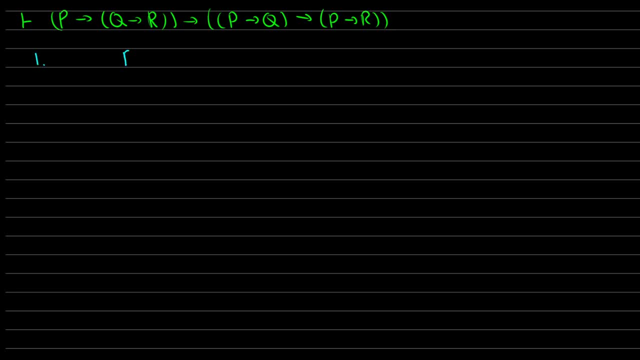 So in line one, I am going to assume p-arrow, q-arrow, r. This is a hypothesis and this is specifically for conditional proof. Who knows how long this has to go. Let's say, Let's say, that's good enough. 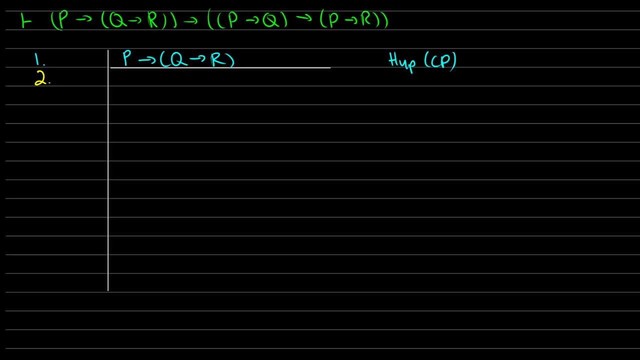 Okay, in line two, I am going to assume p-arrow q- This is another hypothesis and this is for c p. Okay, this one. I don't know how long it'll be. Let's say that's fine. 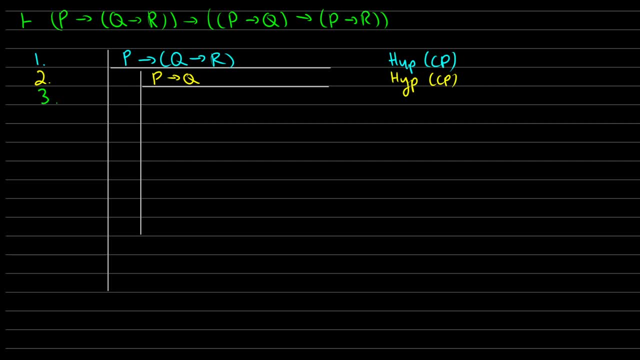 And finally, in line three, what I'll do is I'm going to assume p once again for c, p, c p, having some difficulties remembering what's a bracket and what's a letter. Okay, there we go. 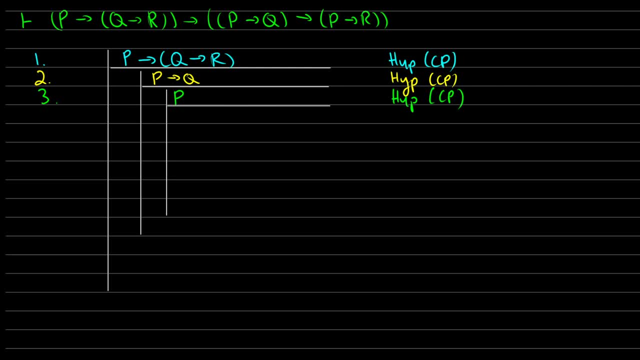 And this will probably take a little up to about here, perhaps. Okay, so we've essentially just assumed all of the consequence that we'll need. So what I'll do now is, in this sub-proof I'm going to reiterate: p-arrow q. 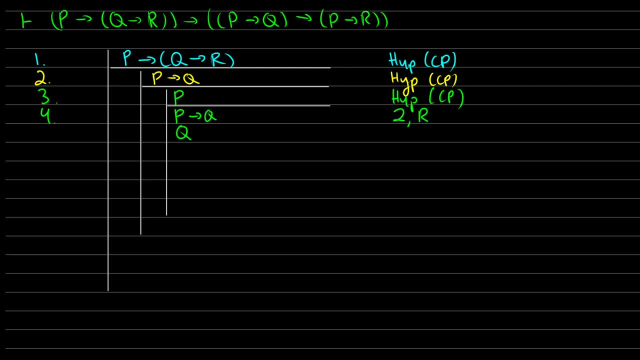 So this comes from line two. this is a reiteration, because that way I can then use modus. So I'm going to use modus ponens on lines three and four to get me q. Okay, but I need to get r in the sub-proof. 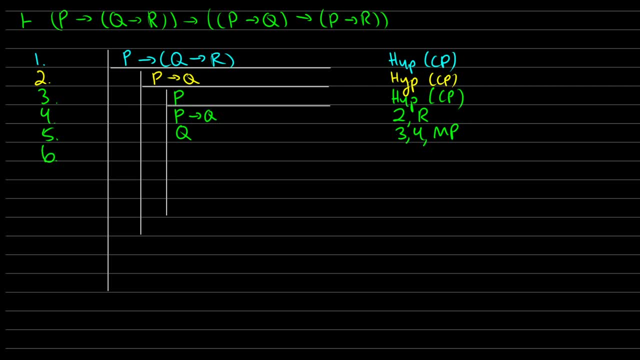 I need to show that if I have p, I get r. So what I'm going to do in line six is I'm going to reiterate line one for p-arrow, q-arrow r, because I can get an r out of this. 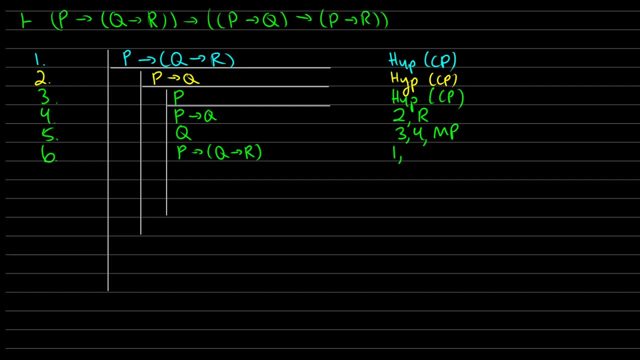 As long as I have a p, as long as I have a q, I can get r. So from line one I'm doing reiteration. In line seven, I'm applying modus, I'm applying modus ponens from line three to line six. so p and then, if p, then q, then r. 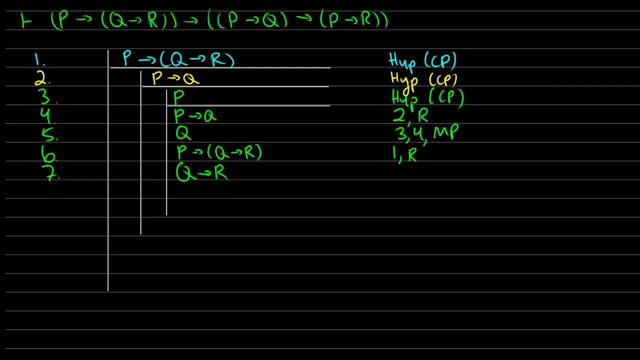 to get q, then r. So this is from three and six. this is modus ponens. Okay, now I can do modus ponens again to get r. I have q and I have q-arrow r, therefore I can get r. 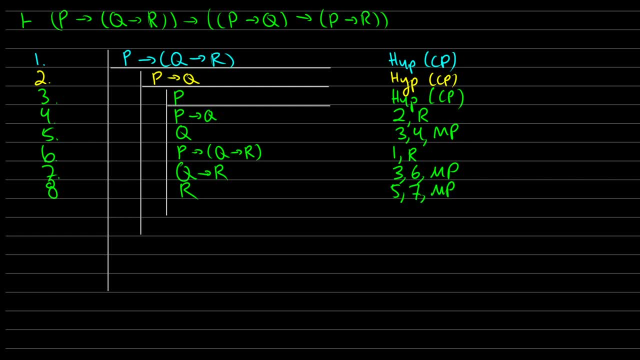 So that is line five and line seven and that is modus ponens. Okay, so now I've shown that if I have p, then I can get r, so I can pull this out using c p. So in line nine we say that from two to or not from two to eight. 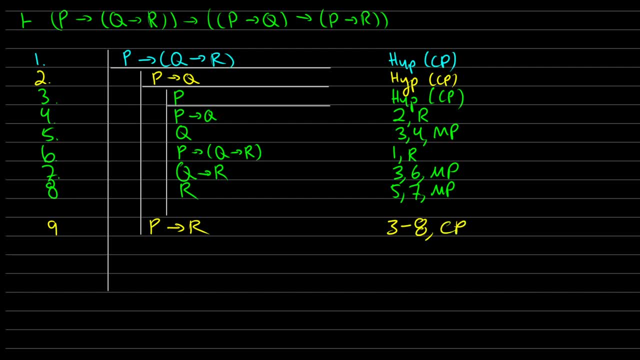 from three to eight. we did a conditional proof. We assumed p. we showed that we can get r. therefore we have p-arrow r. Now in line ten we can do another conditional proof, because we showed that if we have p, then q, then we have p, then r. 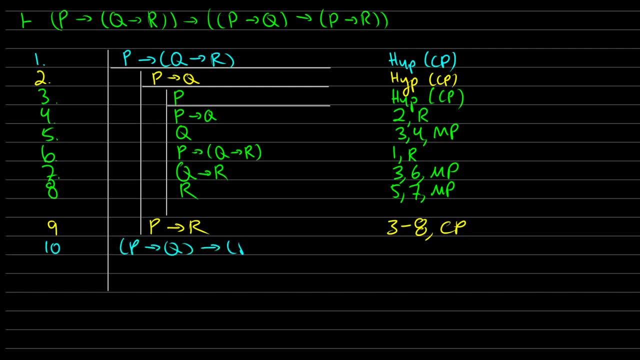 So if p, then q, then r. This is from line two to line nine and this is a conditional proof. Okay, finally, we can now finish this. We can pull this out, because we assumed p-arrow, q-arrow, r. 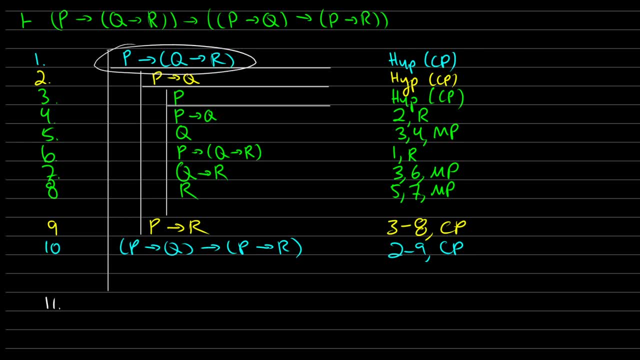 We've shown that, then we get p-arrow- q-arrow, p-arrow- p-arrow r. Therefore, we're going to get that if we have p-arrow- q-arrow r, then we're going to get p-arrow- q-arrow r. 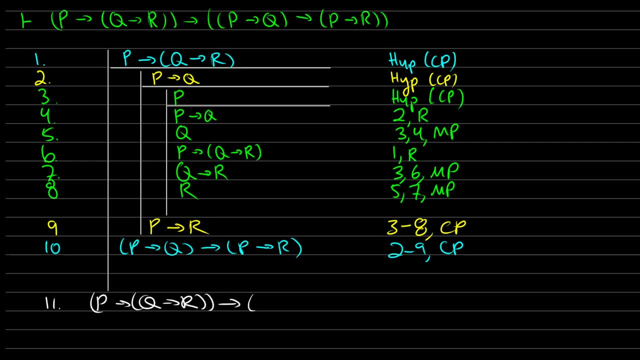 We're going to get p-arrow- q-arrow r, We're going to get p-arrow- q-arrow r And we're going to get p-arrow- q-arrow- p-arrow r. And this is from one to ten and this is a conditional proof. 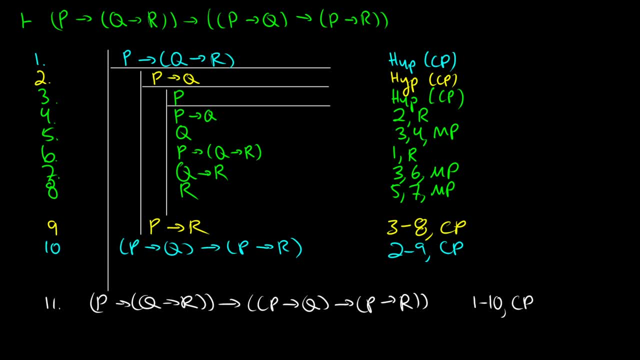 So that would be the proof of p-arrow q-arrow r arrow- p-arrow q. arrow- p-arrow r. So basically, we just keep doing conditional proofs until we get what we want, and we're very lucky that, because these are conditionals- 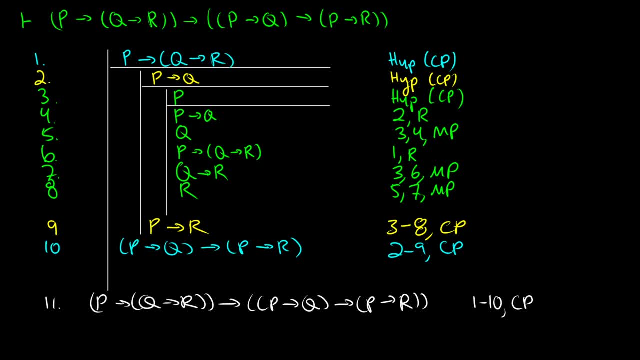 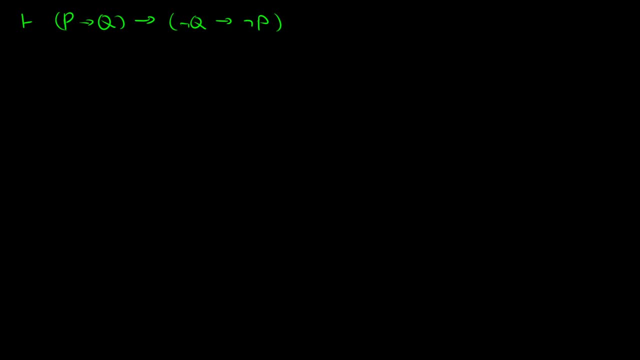 we just have to keep playing modus ponens. So, MPs and CPs, That's the name of the game. when these theorems just have arrows in them, Okay, we'll do one more: p-arrow. q arrow, not q. arrow, not p. 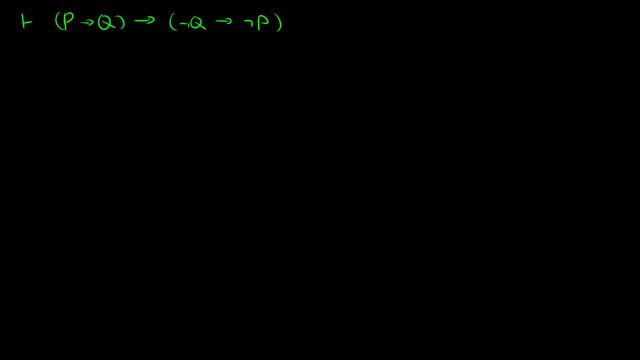 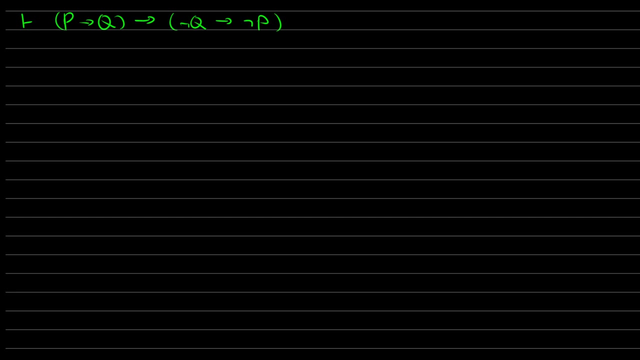 So basically, this just says that the conditional gives us the contrapositive. So we've seen this proof with modus tollens. In fact, we can use modus tollens in this to make this a lot easier. So in line one we're going to assume p-arrow q. 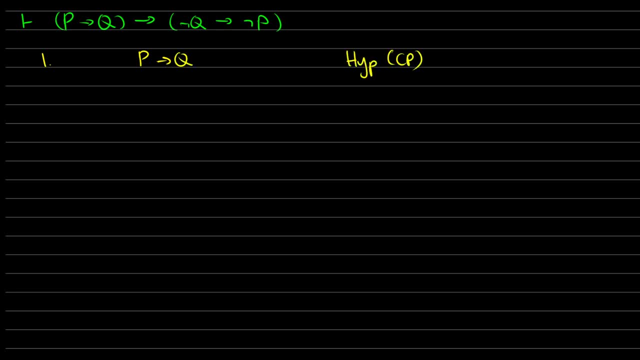 This is going to be a hypothesis for a conditional proof. I don't think this is going to be very long at all, So let's just make it like this In line two: so we've assumed this part. Now we need to assume the antecedent inside the second conditional. 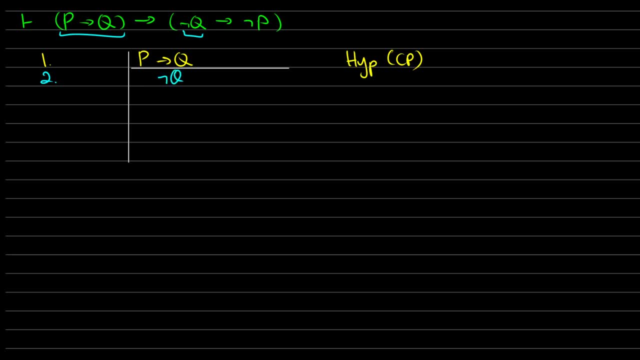 So we're going to assume not q. So it's another hypothesis for a conditional proof. Okay, so what I'm going to do in line three is I'm going to reiterate p-arrow q, so that way we can use it in our sub-proof. 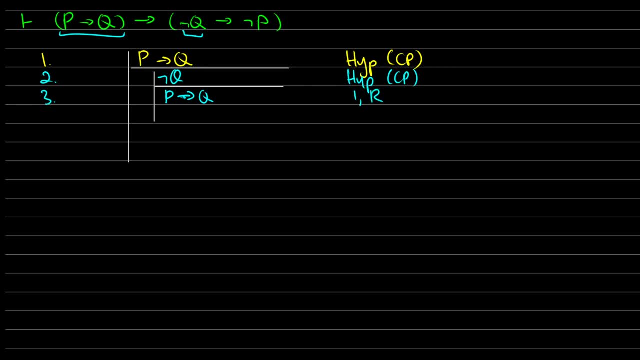 So this is one reiteration, And now I have modus tollens. So, if you remember, we proved earlier that the sequent p-arrow q and not q, let's just say not p. We've done this proof twice in this playlist so far. 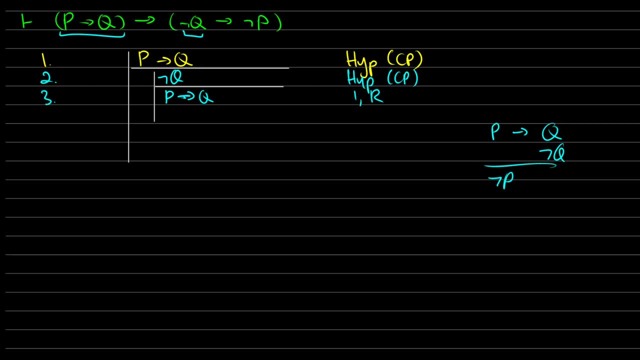 So you can check out natural deductive proofs- number two for that, as well as one of the practice exercise videos I just showed. I think of the derivable rules, Number one or number two is show. Okay, so this means that then in line four, 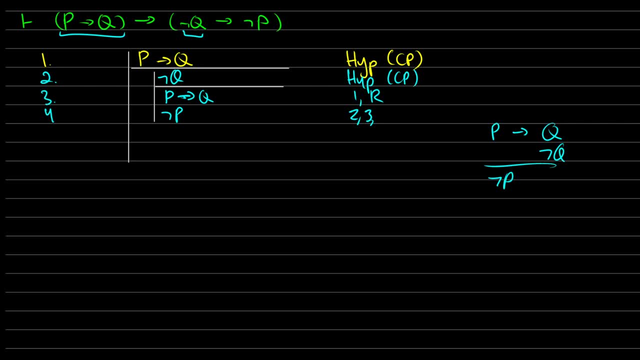 we can write, not p, So this comes from two, three And this is modus tollens, so that's abbreviated mt. If you can't use it again, we have a proof of that in the other videos that you can check out. 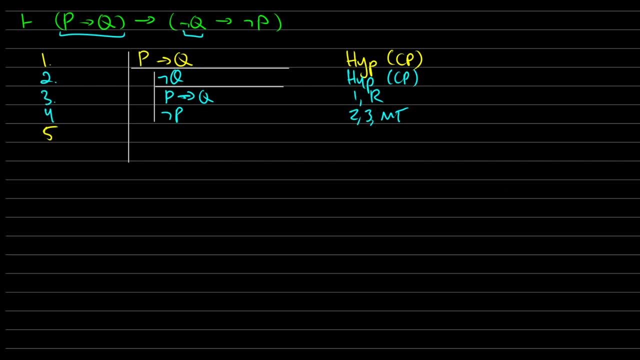 Okay, this means that in line five, we assume not q, we got not p. Therefore we have not q, arrow not p. This is from two to four, And this is a conditional proof, which means then that in line six, 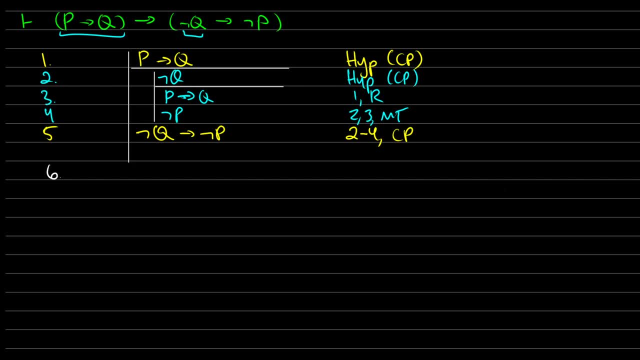 well, we assume p arrow, q From that. we got not q arrow, not p. So we can use the conditional proof to say that if we have p, then q, then we have not q, then not p. 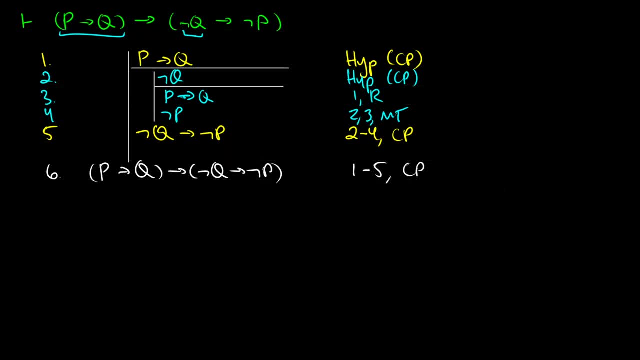 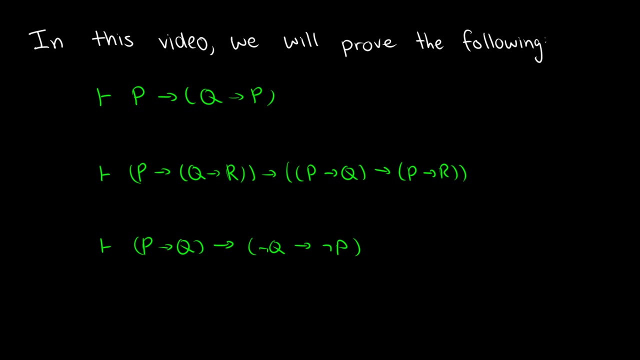 So, from one to five, this is a conditional proof And that is the proof of p arrow, q arrow not q, arrow not p. So what I want to show and what I want to say is that these three things. 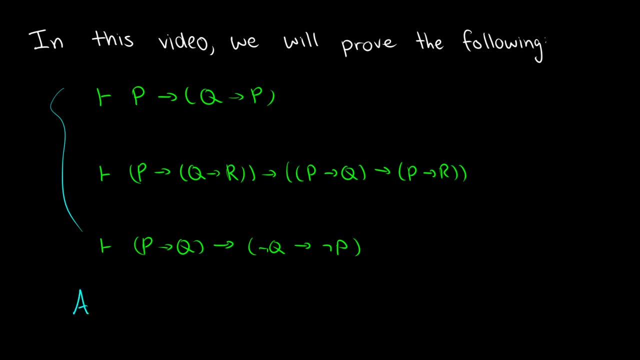 these comprise three axioms, So some systems would call- I should really be more specific- this one a1,, this one a2, and this one a3.. And basically from these three, along with the contradiction symbol, the arrow, and p's and q's.